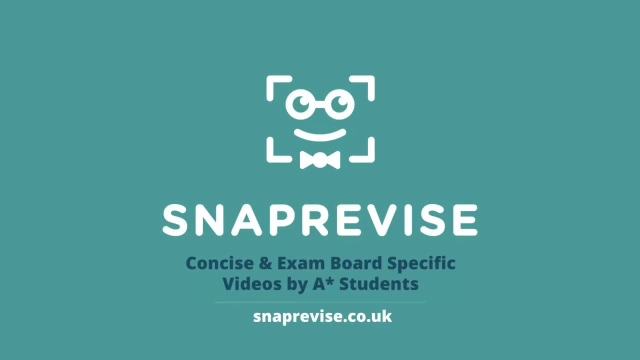 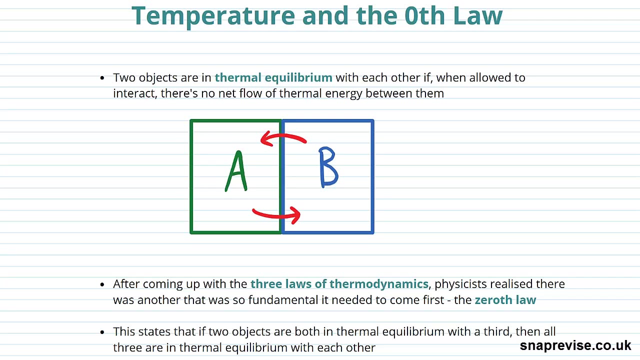 So now we're going to go back to thinking about one of our laws of thermodynamics and we're going to look at how it applies to temperature. So we're going to first off say that two objects are in thermal equilibrium- which might be a phrase you've heard before- might not be with each other. 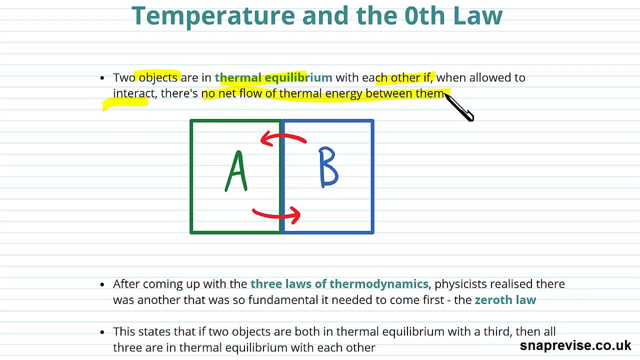 if, when allowed to interact, there's no net flow of thermal energy between them. Now, to be clear, allowed to interact can mean kind of anything, as long as it just means that it's just these two systems involved and they're allowed in some way to exchange heat with each other. Remember, you can. 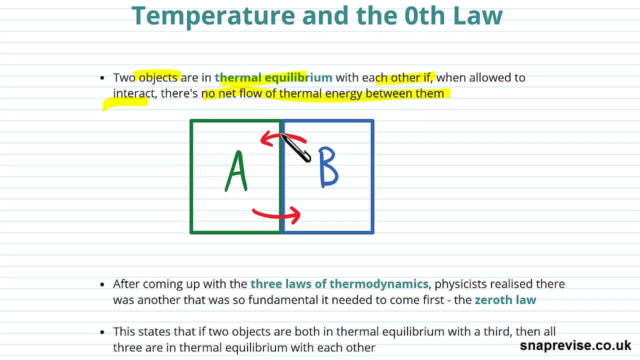 do that in a vacuum, through radiation, etc. There's plenty of different ways for you to exchange heat. You could do it by conduction, convection, radiation. The key thing is that you have to have some way of interacting. We say in thermal equilibrium, if there's no net flow, There will. 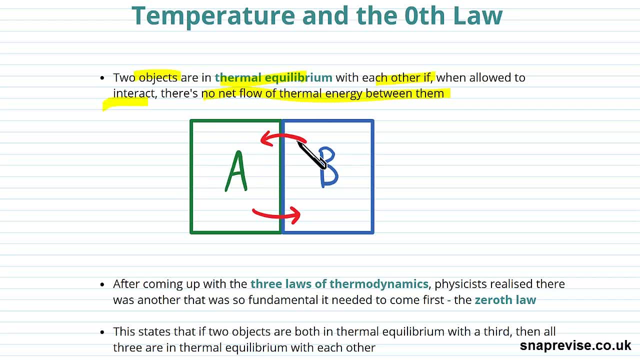 still be. you know, it's still possible to exchange thermal energy, but what will happen is that whatever this one gains, this one will then gain back. It's going to be a net flow. It's not going to be that, for instance, if they're not in thermal equilibrium. it means that this arrow 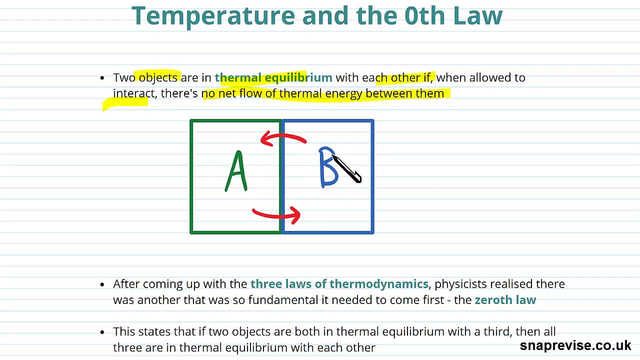 would just go one way. On balance, there would just be a net flow, Thermal energy moving from here over to A, for instance from B to A. But if they're in thermal equilibrium, there's no net flow. That's the definition. 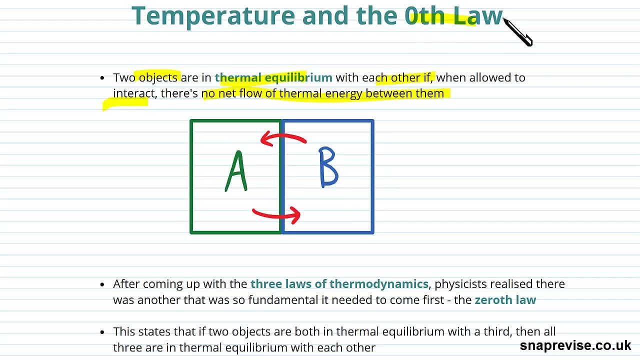 So why would we call it the zeroth law? Well, because after coming up with three laws of thermodynamics, physicists kind of realised that there was another thing like so fundamental underpinning everything they were doing. that kind of needed to come first. but they hadn't. 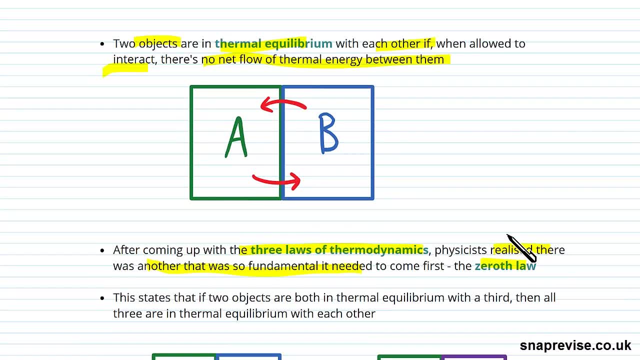 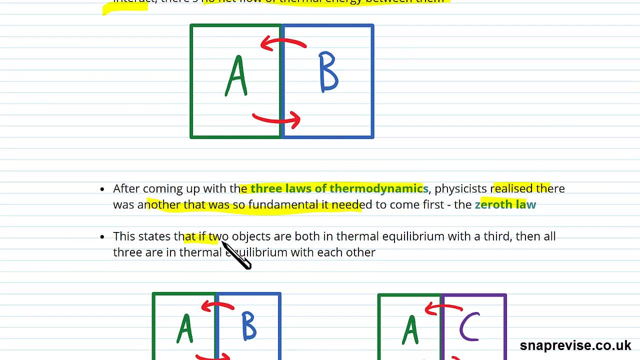 explicitly given it a law And so it became the zeroth law. And this kind of just is very simple and it just uses this definition of thermal equilibrium And it really just states that if two objects are both in thermal equilibrium with a third, then all three are in thermal equilibrium with each other. And you know that might. 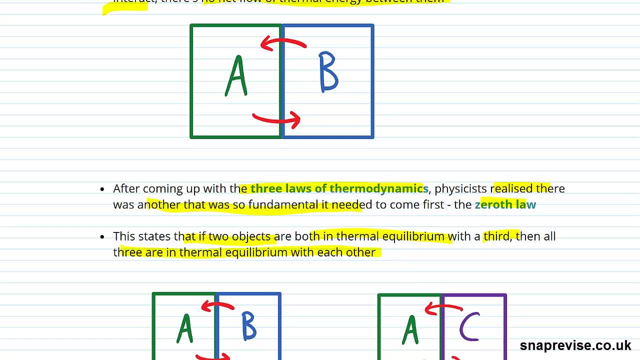 seem really obvious, but it is really crucial as well. So just to make clear what I'm talking about there, let's say, just as we've got here this A and B exchanging, let's say now we've got an A and B and an A and C. 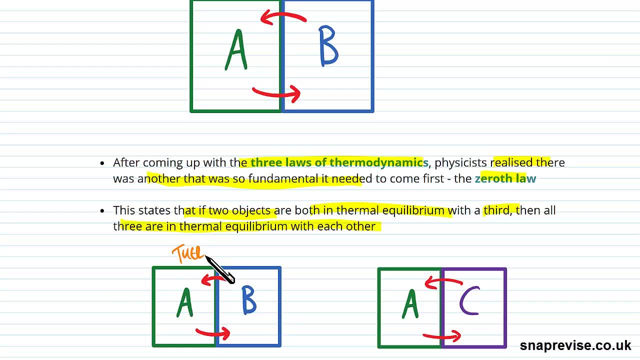 We're saying: these A and B are in thermal equilibrium, That is to say, there's no net flow. We take A Wherever we've got A from, we bring it in. And we take B from wherever we've got B from and bring it in. And what we say is that when we put them next to each other, they don't.